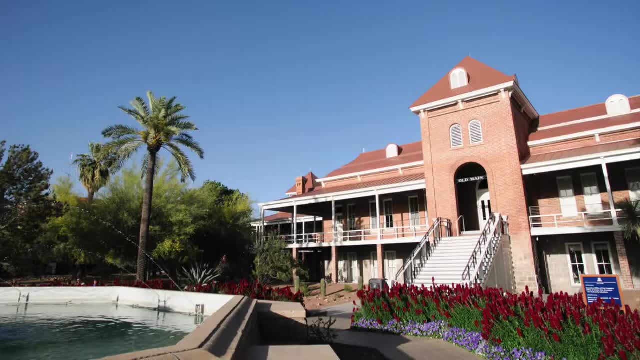 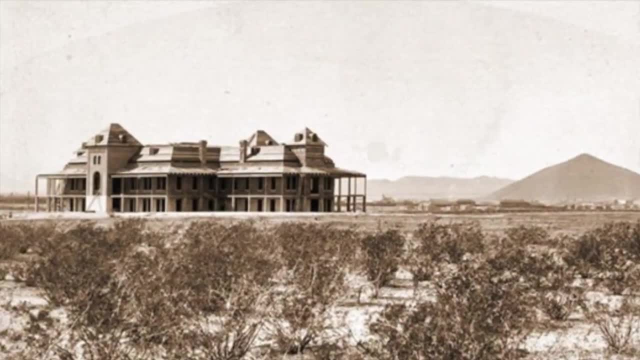 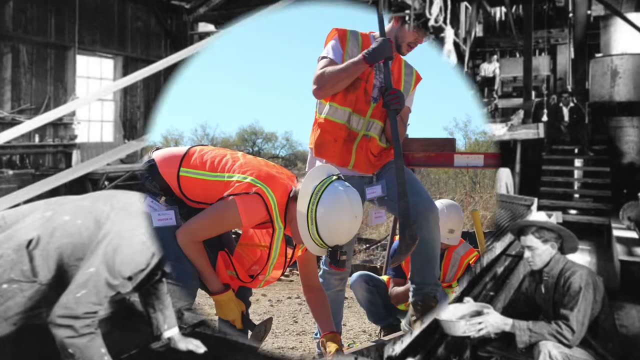 The University of Arizona is one of just 13 American universities to offer a mining engineering degree. The program stems all the way back to the founding of the school and was the very first program to be established here, back in 1885.. Of course, a lot has changed since then, but one thing that has remained is the program's. 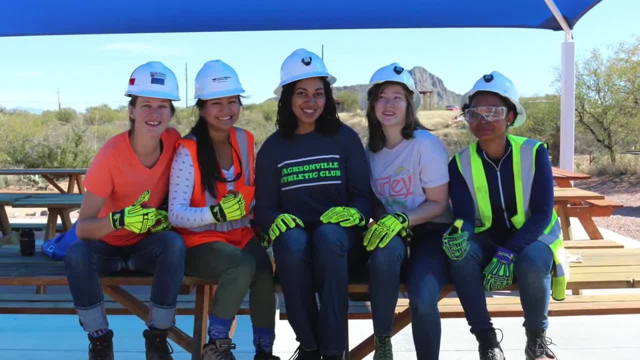 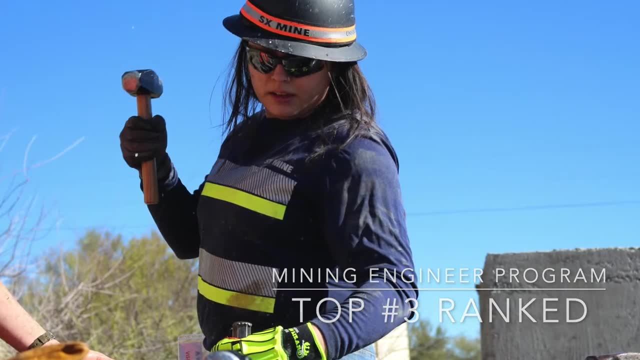 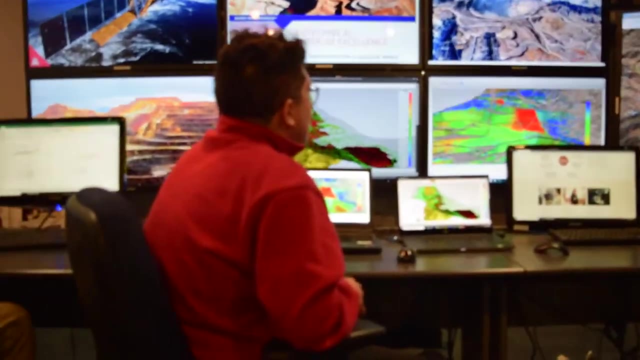 long tradition of excellence as a leader and innovator in the field. In fact, the program has been consistently ranked as one of the top in the world in the nation, year to year. University of Arizona. mining engineers make a global impact by solving the critical challenges. 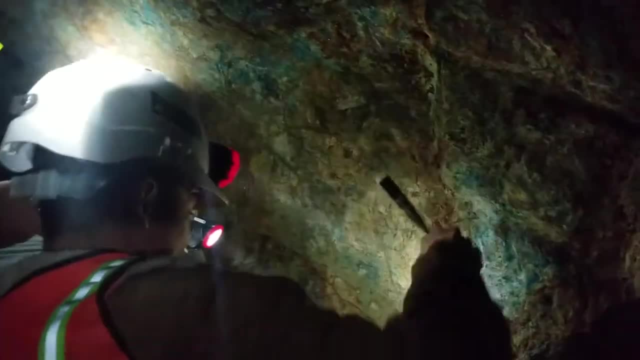 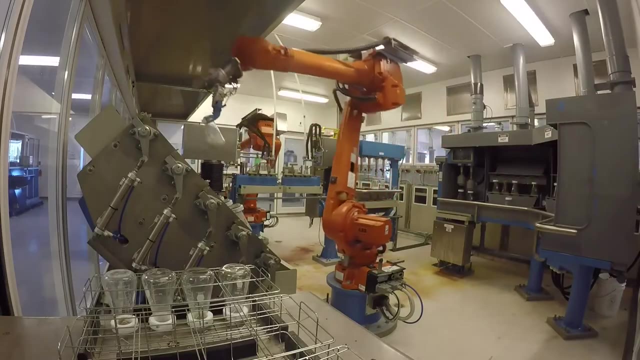 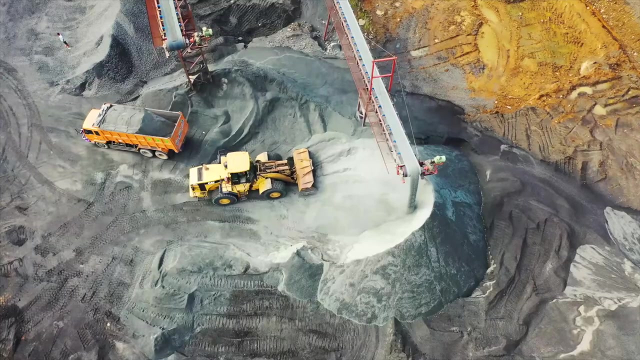 of extracting non-renewable natural resources, processing them and turning them into the materials necessary to create the things that we need. Cutting-edge technologies like battery-powered vehicles, solar panels or life-saving medical devices all rely on mining engineers finding new ways to extract more complex minerals. 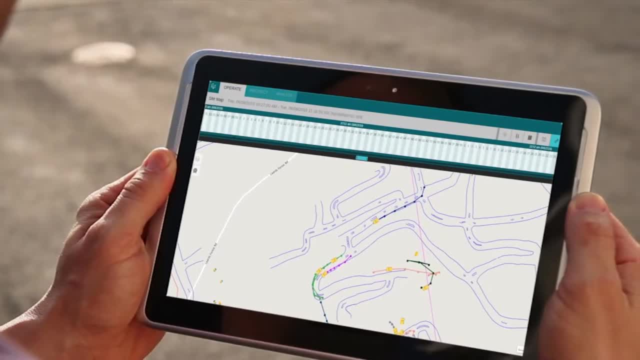 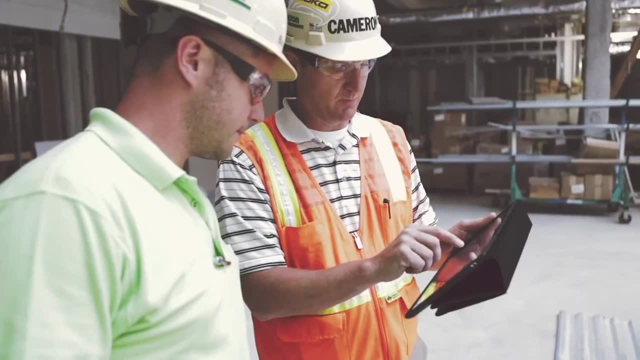 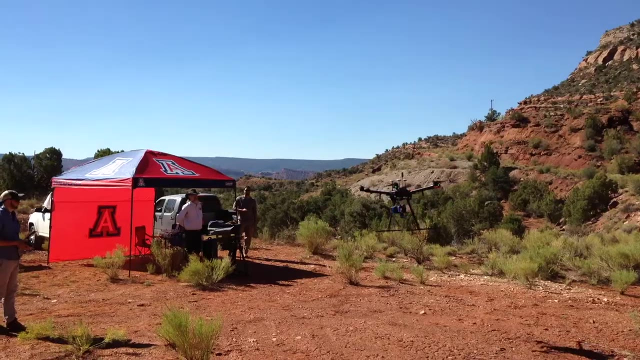 in lower concentrations, developing new technologies and making sure that the process is done in a safe, socially responsible, environmentally sound and economically viable manner. The program here at the U of A is designed to give you a strong mining engineering foundation, while also allowing you to discover and pursue your own passion. 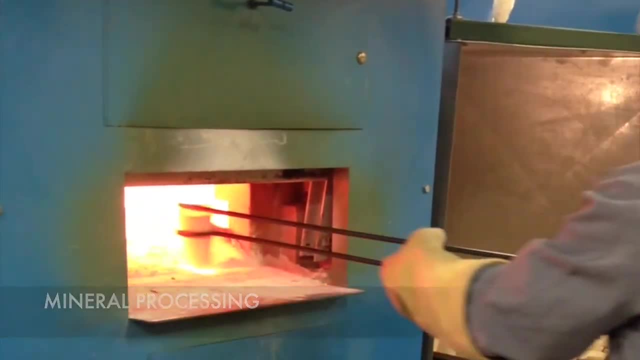 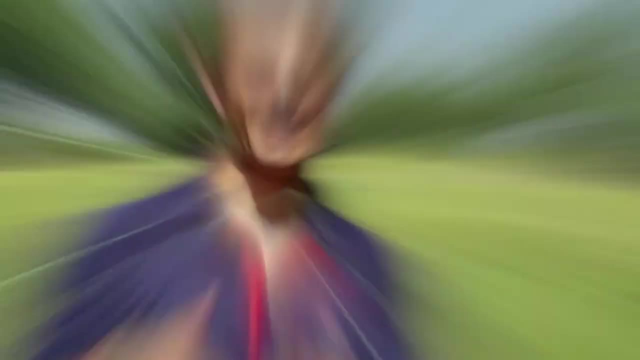 With four different focus areas or tracks to choose from, you can really dive into what you find most interesting and take the courses related to that topic. Thank you. Having been through the program myself, I can tell you that one of the things I found- 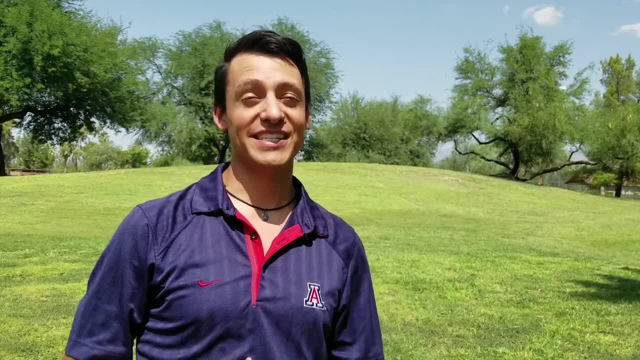 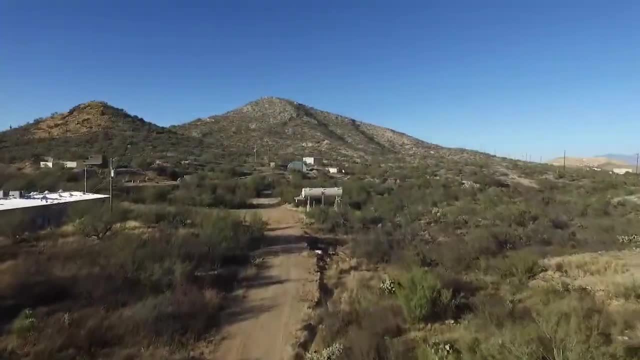 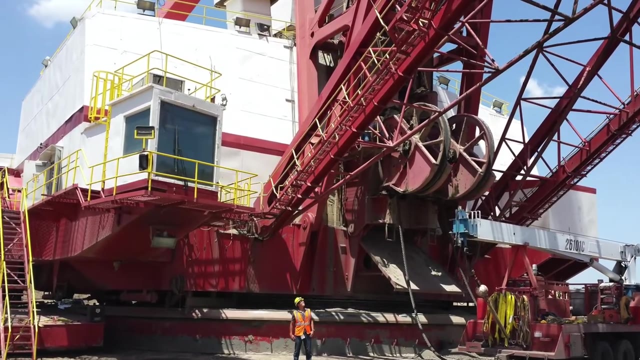 most exciting about it was the plethora of opportunities to gain hands-on experience and get involved, Whether it's working underground at the San Javier Mining Laboratory or assisting a professor with cutting-edge research, or even working and getting paid as an intern with one of 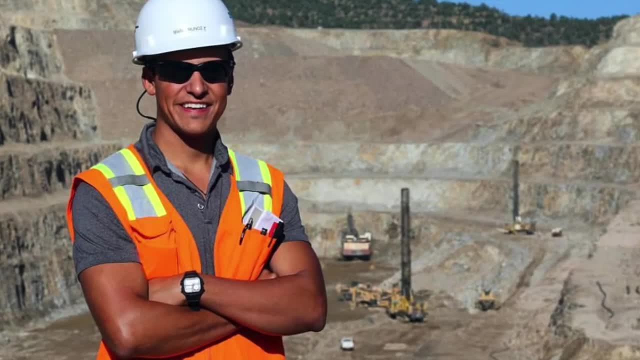 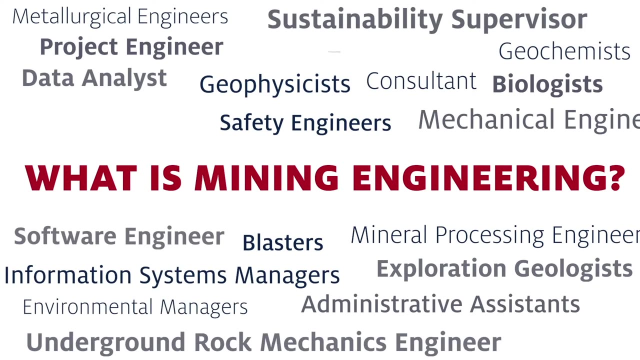 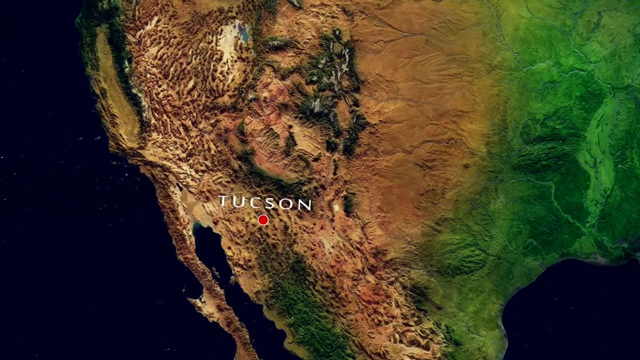 the local mining companies. there's so many ways that you can gain practical experience. Believe me when I say that there are truly so many different career paths a mining engineer can take. Tucson alone is a mining hub, surrounded by mines, consultants and mine technology companies.